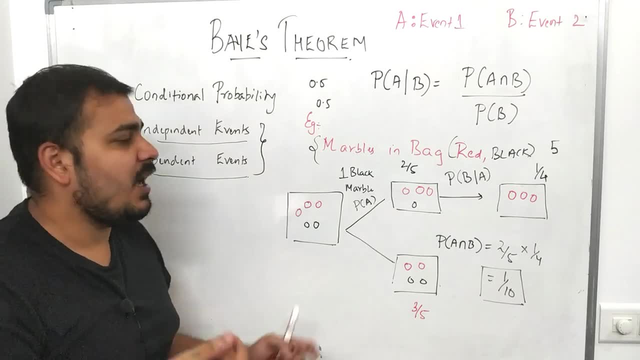 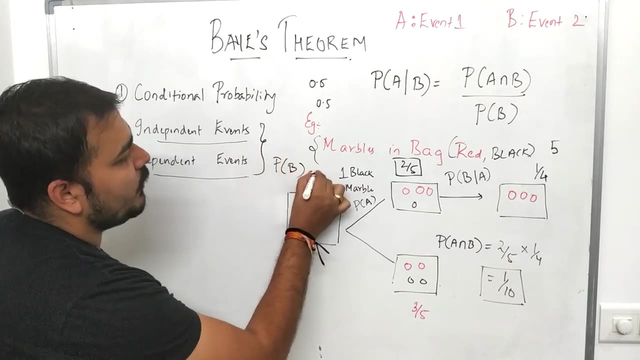 be the probability of getting this black marble, black colored marble. It will be somewhere around two by five, Right? So the probability of getting a black marble will be two by five. Why two by five? The total number of marbles are five And you can see that out of two right, these two black 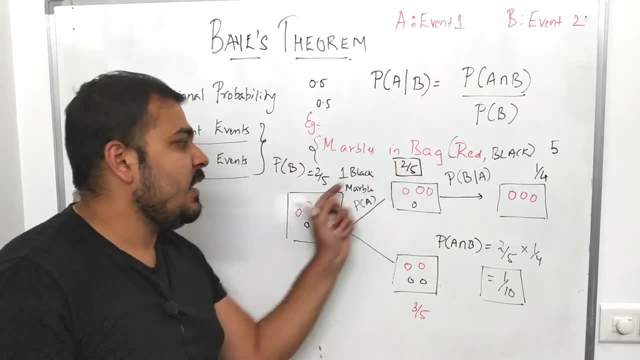 marbles are there. So I can basically write two by five. So this will be the probability of getting a black marble. So I can basically write two by five. So this will be the probability in the first event of taking out the specific marble Now. in the next, 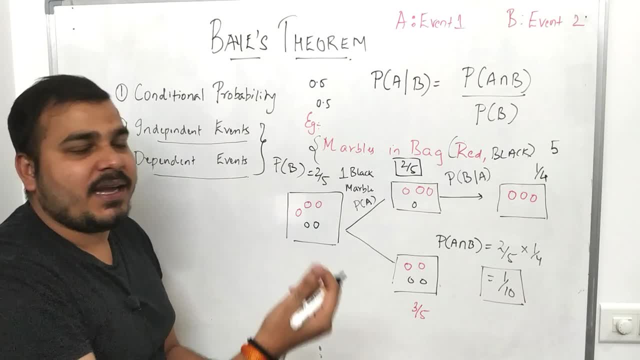 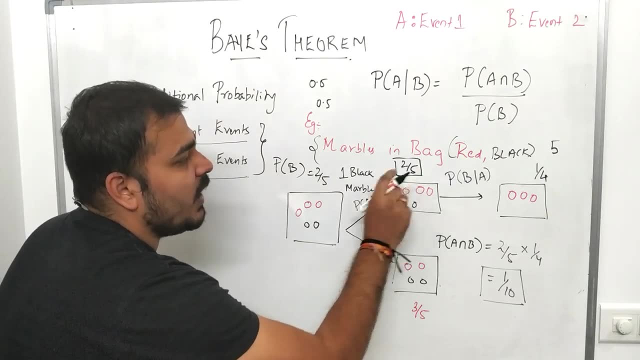 event. suppose, if I go back to the next event, In the next event again, if I want to pick up one marble out of these four- because one black marble has already been picked up right now out of these four- if I try to pick up one more black marble, then what will be the probability? Right? 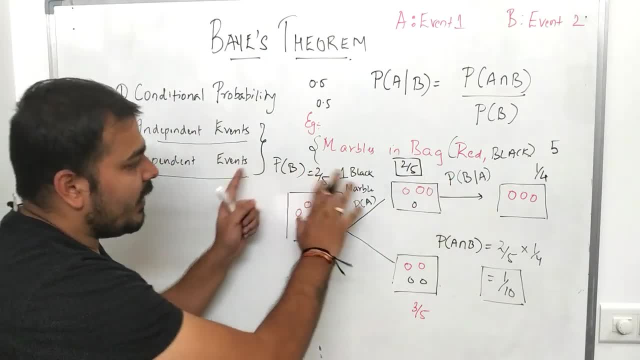 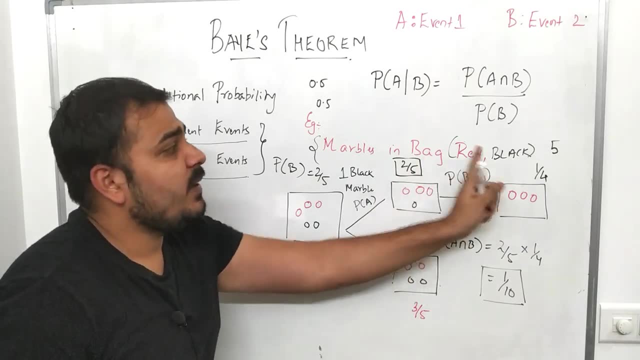 now this is just like an independent events Right over here. one event is there. we have actually picked up a marble. Then again in the second event, from the remaining marble we are picking it up, Then the probability will be changing. It will not be the same as we saw. 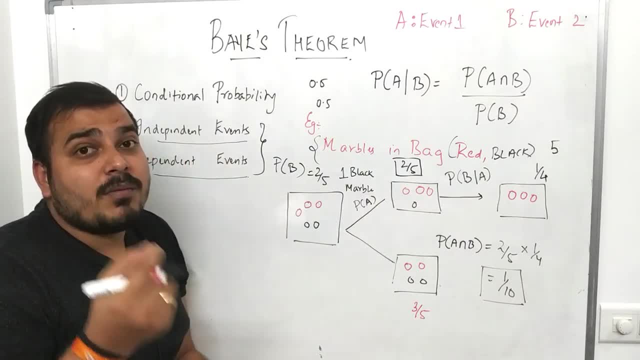 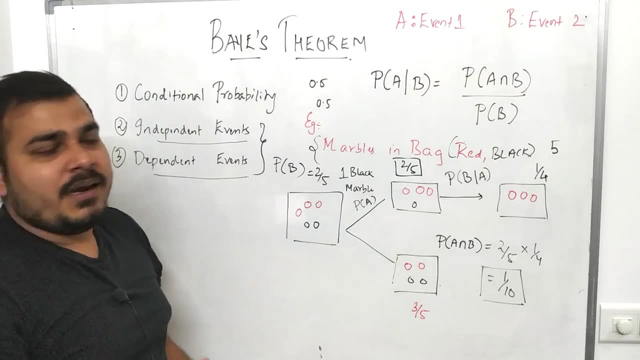 in the independent events, where the probability was 0.5. But in this case, the probability keeps on changing because the number of marbles is becoming less. This was one example of dependent events. Now let us go ahead and try to understand what exactly is conditional. 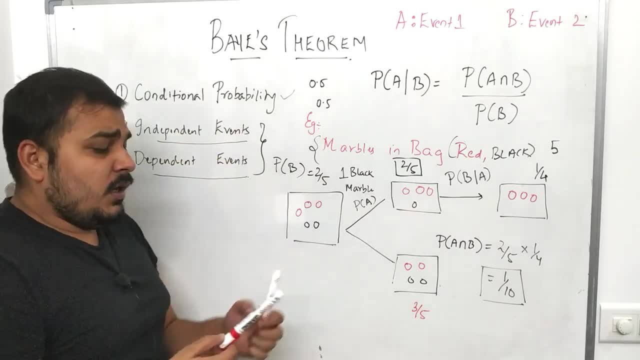 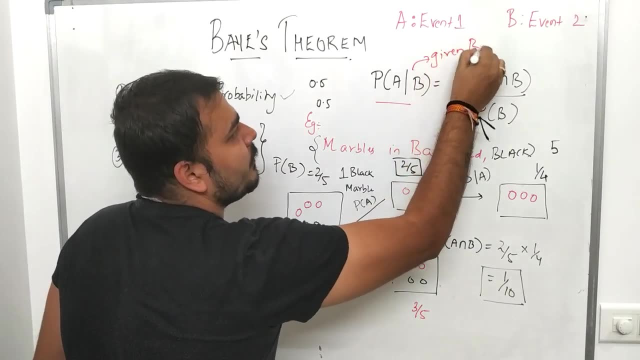 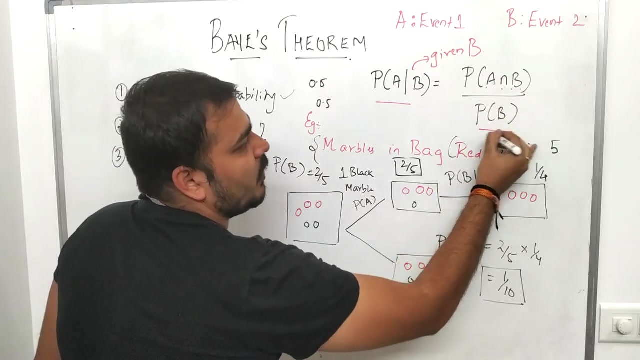 probability. Now, conditional probability is basically given by the formula probability of A given B, and this is basically given by probability of A intersection B, X. probability of Bいる A zhōrprīy is given by probability of A zhōrprīy of B divided by probability of B. I will try to understand thisivelyAKB. 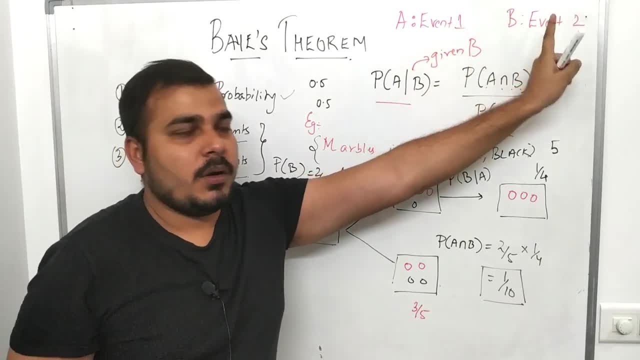 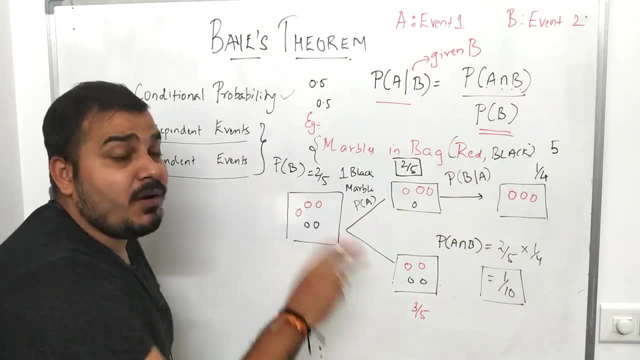 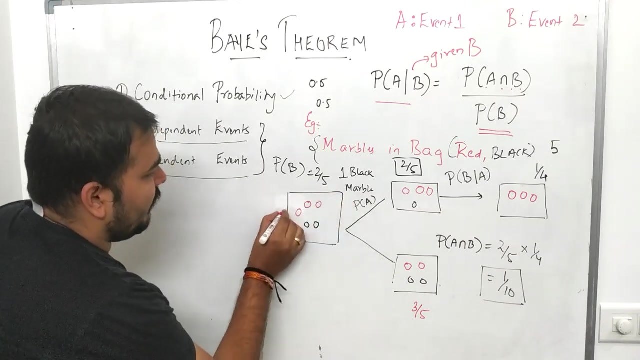 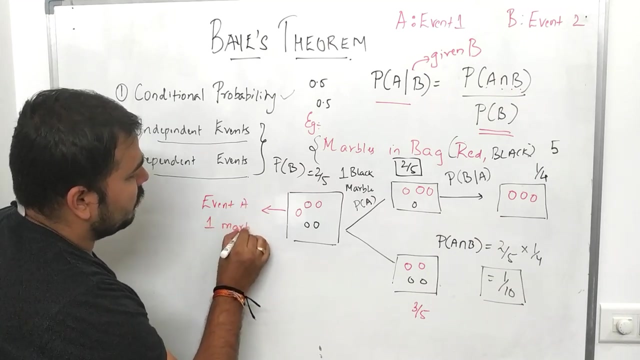 is a and B are two events, event one and event 2.. OK, Now let me just consider the same example. Suppose I want to find out what will be the probability of taking two marbles, with one event continuously after the other. okay, so suppose in event A I have picked up one marble. okay, and this? 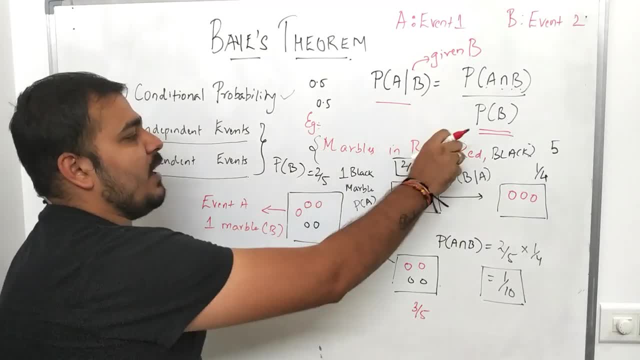 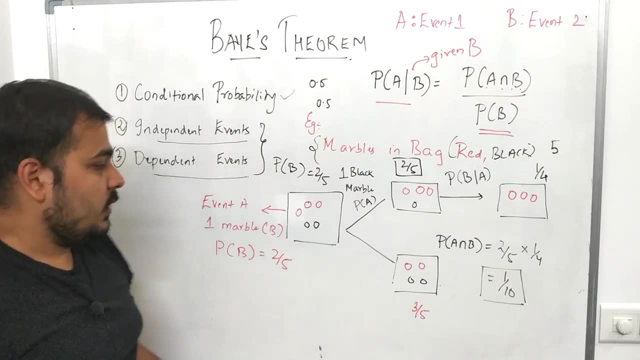 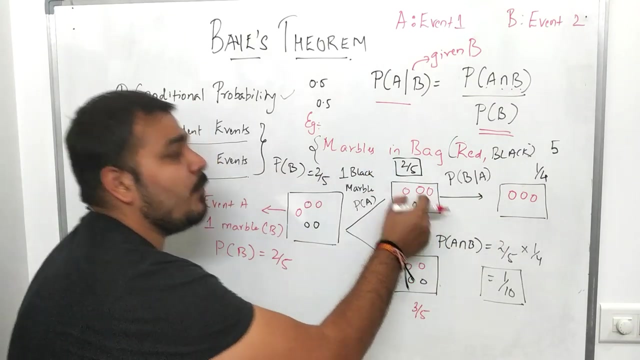 particular marble is of black color. okay, so when I pick up one marble, the probability of this black color is basically 2 by 5. right now, in the second event, again, we want to find out what will be the probability if I take out one more black marble from here. okay, so, 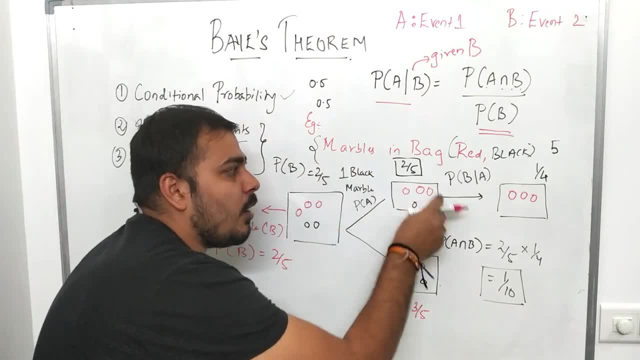 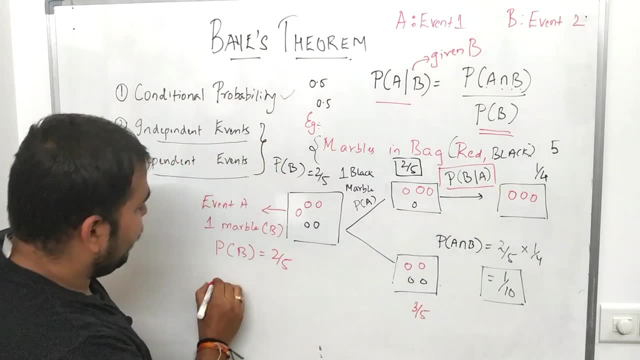 I'm taking out one more black marble from my bag, so what will be the probability that I will basically be getting so for this we can actually indicate this type of equation. so we will be saying probability of B. that is the second black marble, which is my second. 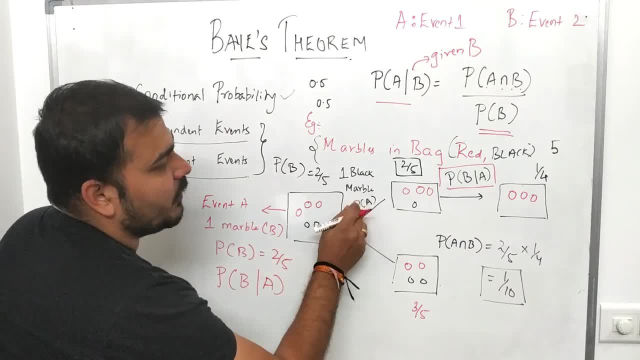 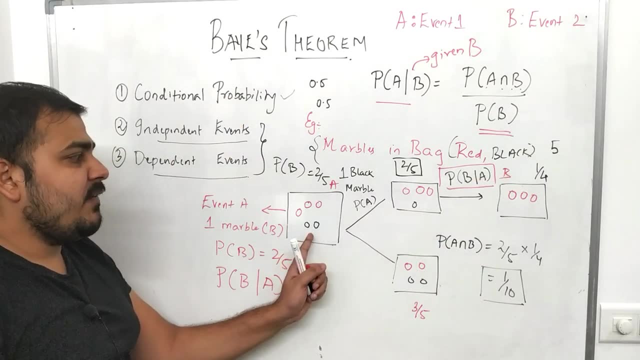 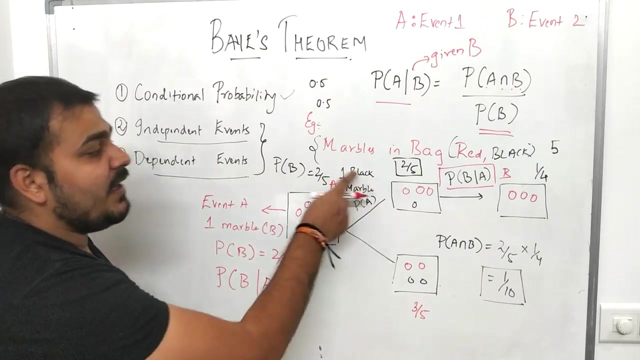 event given already A event is performed. right, this is my A event. understand this, guys. this is my A event. this is my B event. Okay, in the A event, I have already took out one black marble. okay, so I will basically write probability of B, given A event has already taken place. now for this, we basically get. 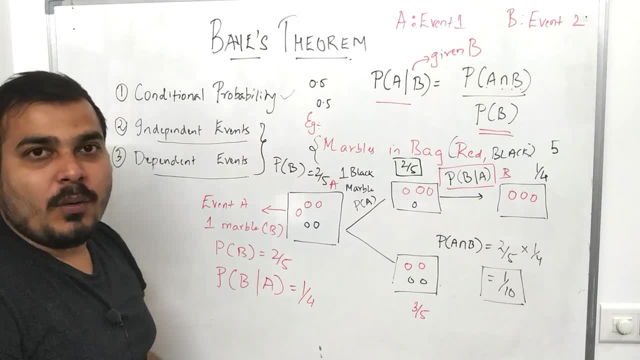 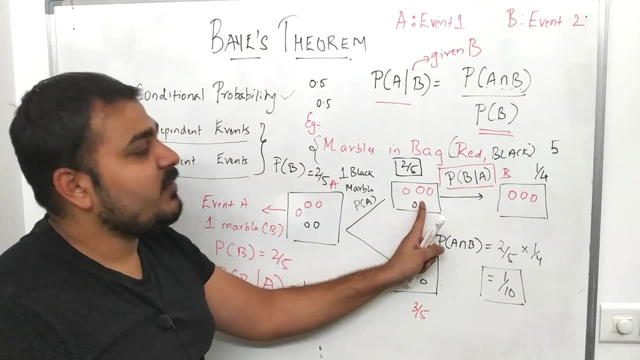 a value 1 by 4. right, 1 by 4. here you can see right in the first event the probability of A is nothing but 2 by 5. in the next event, if I want to again pick up this black marble, the probability will be nothing but 1 by 4, because one black marble is there and total. 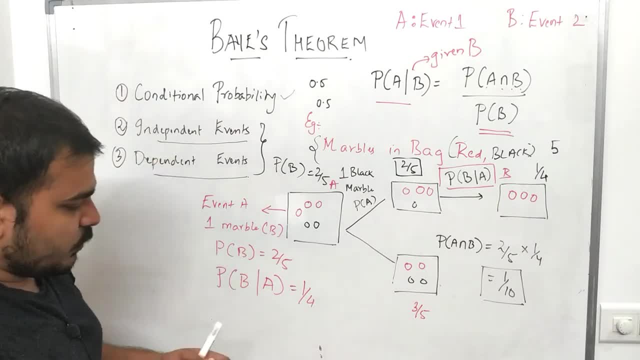 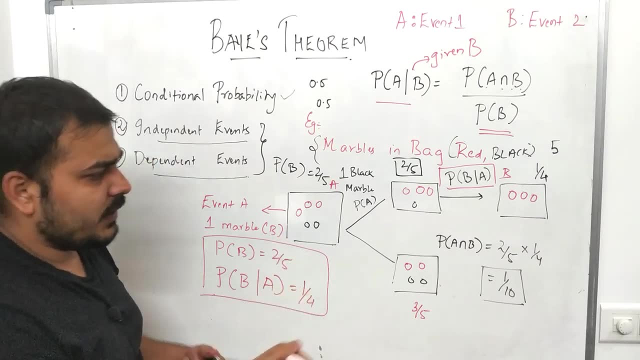 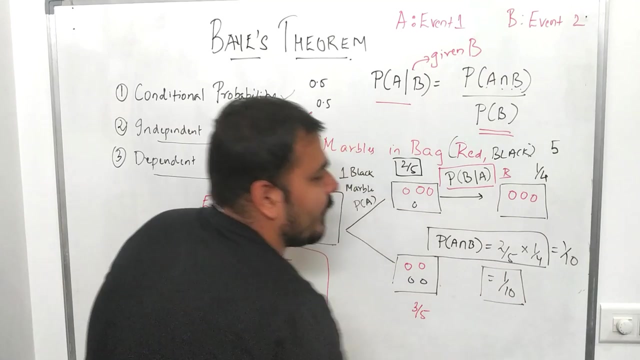 number of marbles are 4 right Now when we are considering the probability of A. we have already taken out one black marble in this, when we are actually considering this right. if I try to multiply both this right, so if I try to multiply 2 by 5 and 1 by 4, I will be getting somewhere around 1 by 10. 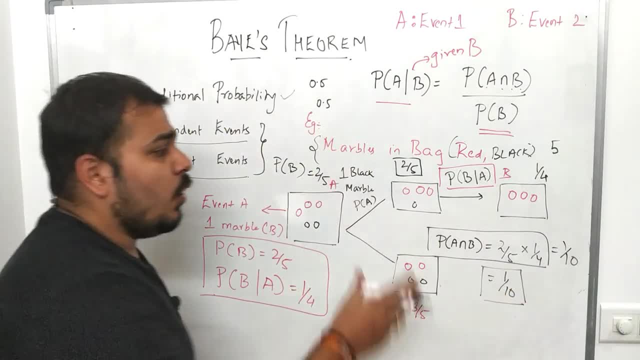 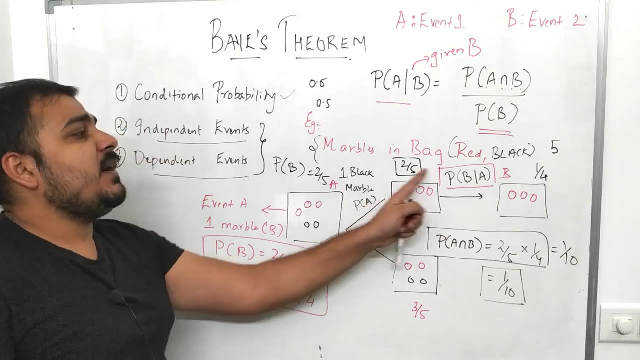 now, what exactly is 1 by 10? 1 by 10 basically says that what is the probability of both A and B event taking place, and that can be only told after this particular event has taken place. So over, here we are combining this particular probability. 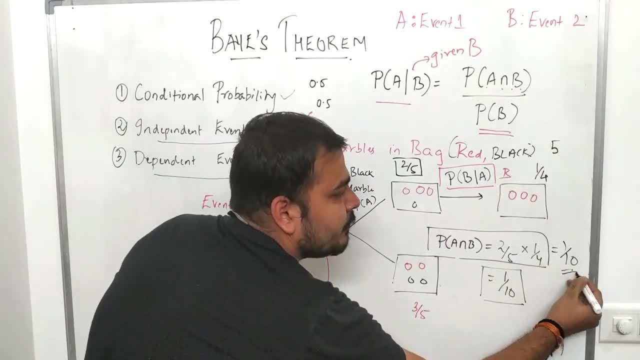 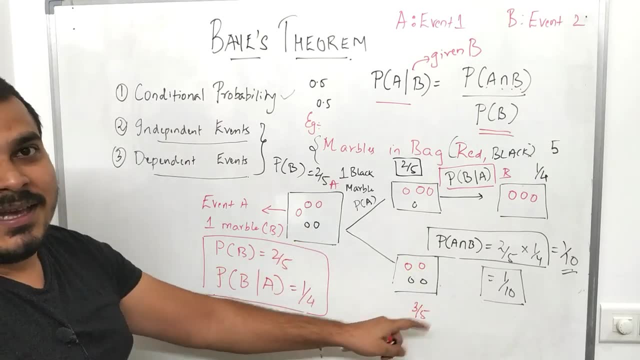 2 by 5, multiplied by 1 by 4, and we are getting it 1 by 10. right now, just understand, guys, if I consider this equation and if I consider all these things that we have done, is it matching or not, how I am saying it is matching or not. just consider that. I will write probability. 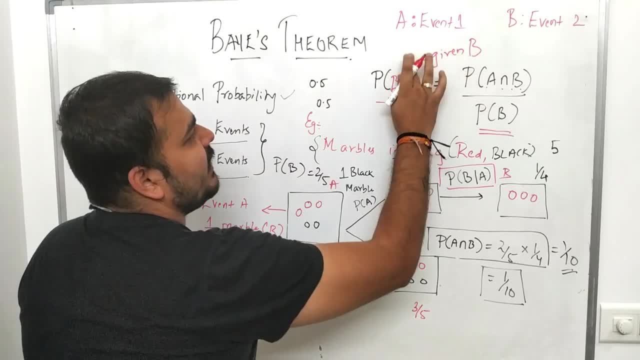 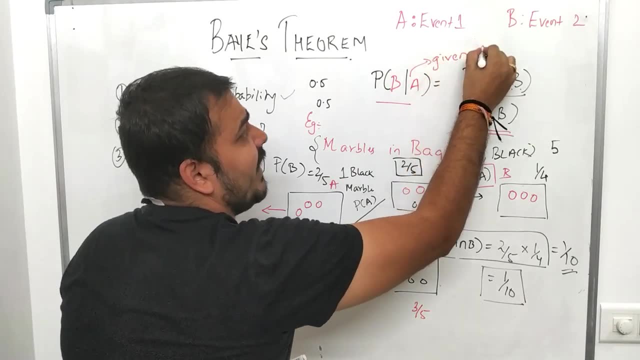 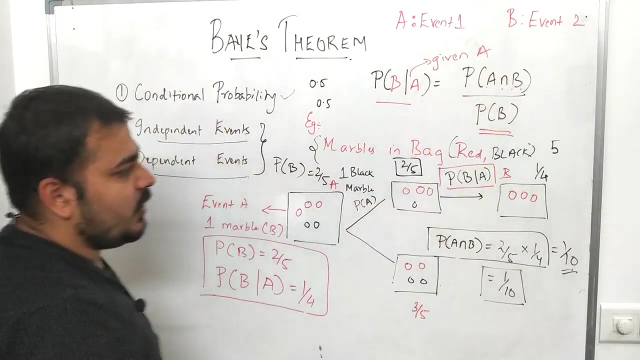 of B slash A. this basically says that what is the probability of the B event, considering or given A event? that basically means A event has already happened, right? so probability of A intersection B Divided by probability of B- right, we know. probability of A intersection B is what? 1. 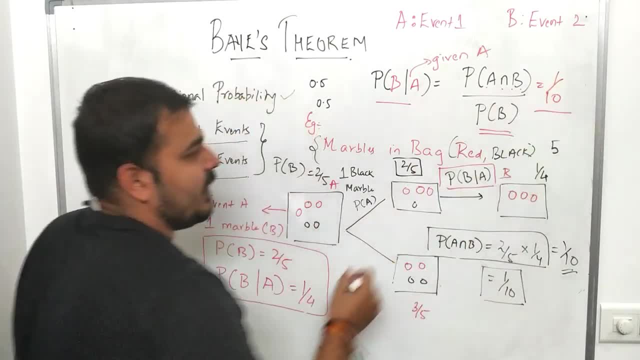 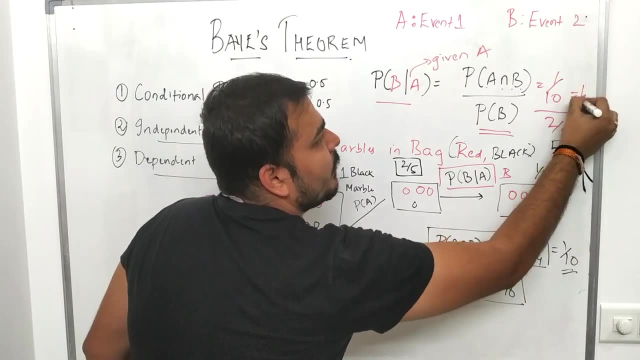 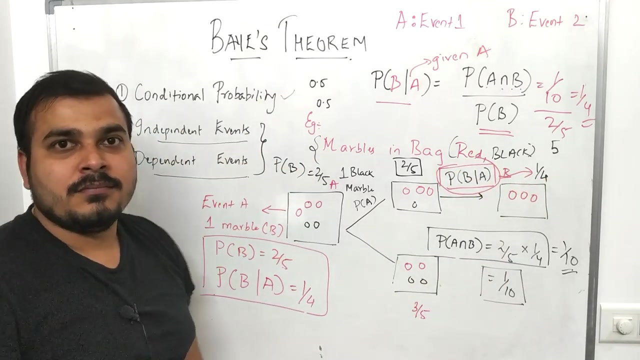 by 10 and divided by what is probability of B, 2 by 5 right now. if I take this down, this will nothing be. it will become 1 by 4. now, here you can see that probability of B by A. the probability that I got is 1 by 4, right, so this is amazing. you can see that based 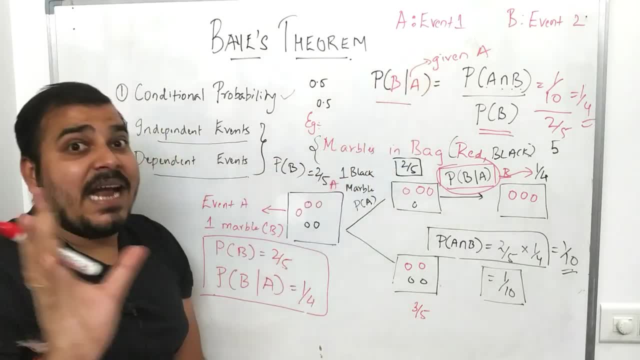 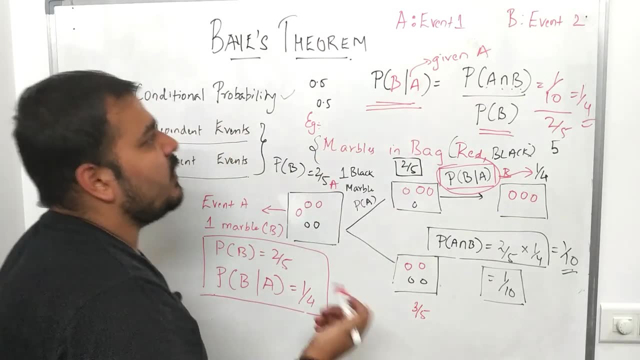 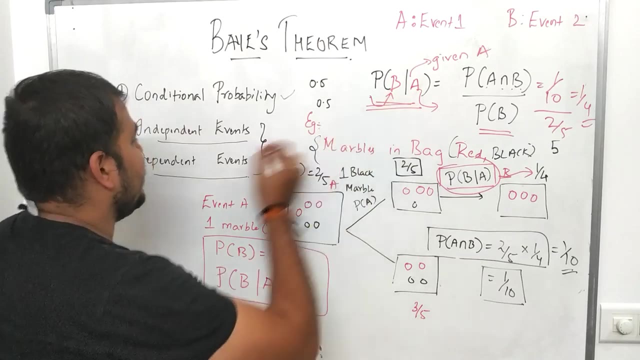 on this conditional probability you need to understand. I will tell you the exact application of conditional probability just in a while, but just understand that. what does conditional probability say? it says that you are trying to find out the probability of an event, given this particular event has already taken place, right? so this is a kind of dependent events. 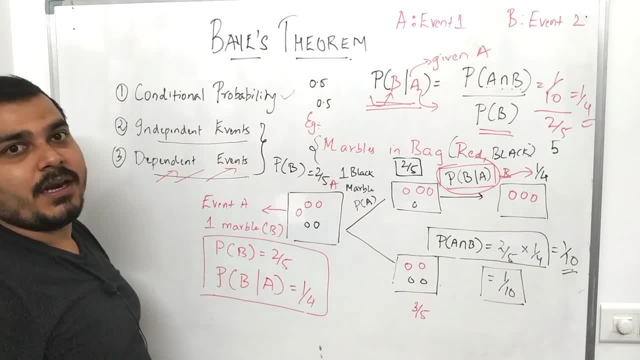 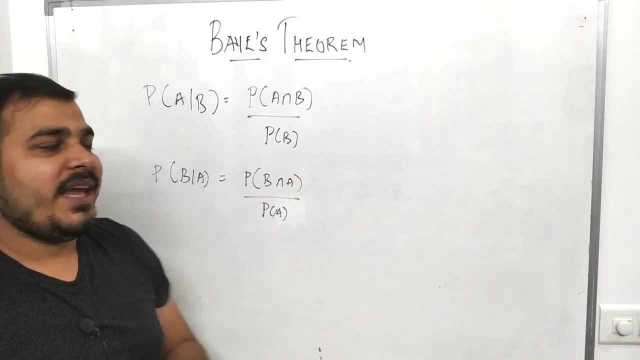 it is not independent, it is dependent always. remember, in this particular way- and I had actually shown you this particular Marvell problem- I had also defined or find out some of the values. so this was just an example. okay, now how this conditional probability, useful for deriving base theorem, will try to understand. now guys will try to take this. 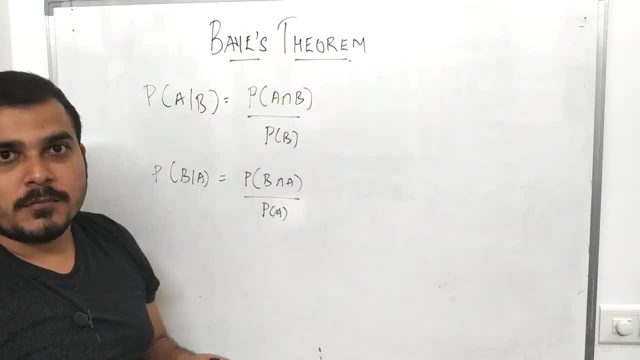 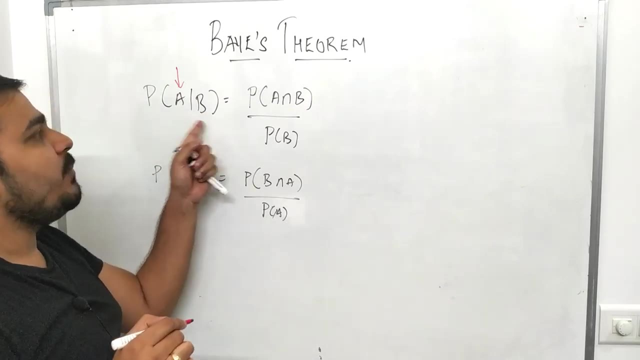 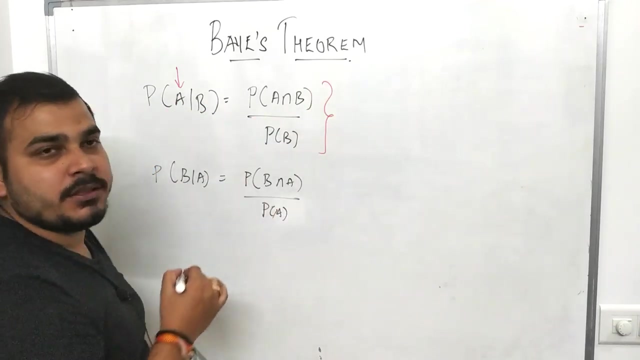 particular conditional probability and will try to derive this base theorem. now just understand over here. suppose if I say that I want to find out the probability of the event A considering B is already given right or B is already happened, this particular event has already happened. so for this we can basically write this kind of equation similarly for the next conditional. 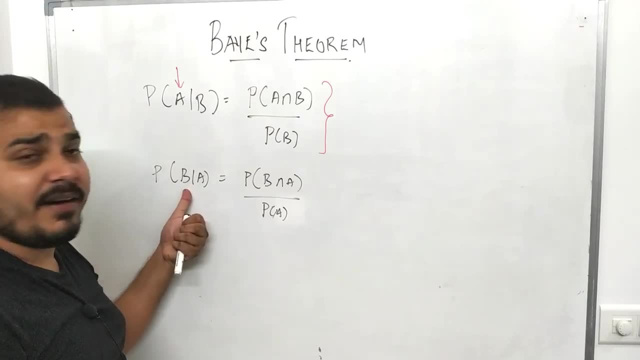 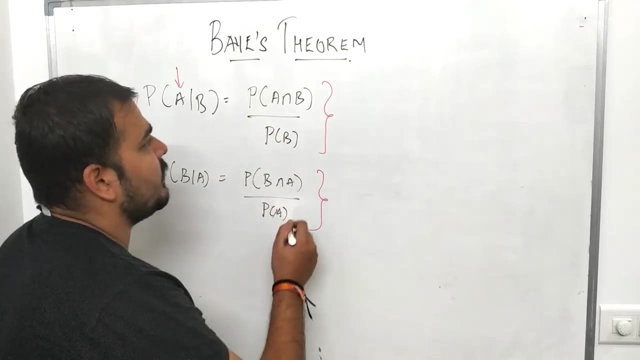 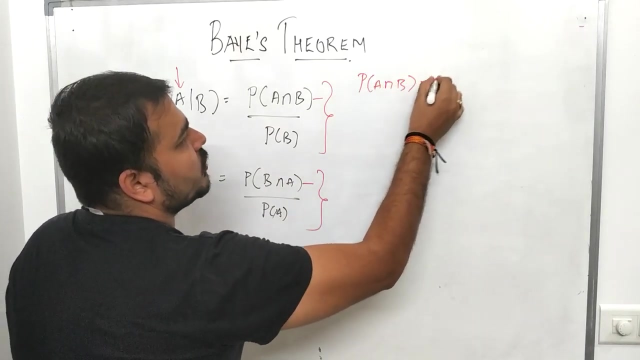 probability. I'm saying that try to find out the probability of B event given. A is already given over there. So if I consider that this will be my another equation, now understand one thing, guys: this value and this value are almost same. I can also write it as P A intersection, B- P B intersection. 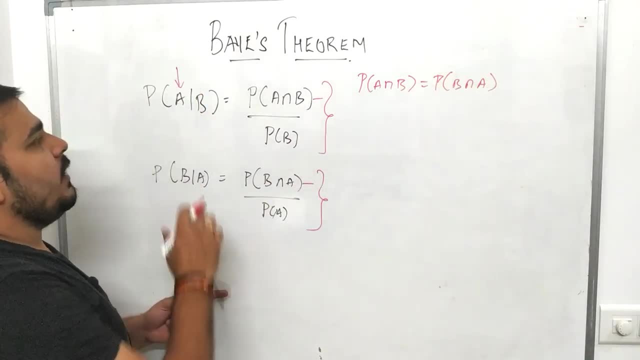 A. it is both equal. they both are actually equal, okay. so what I'll do? first of all, I'll just, you know, take this denominator and put it on the left hand side. take this denominator and put it on the left hand side, so this will basically become P A. intersection B is equal. 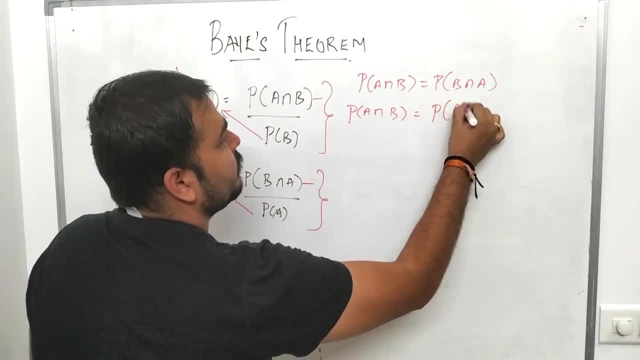 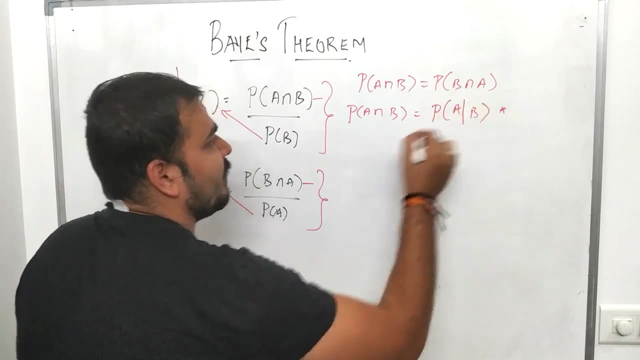 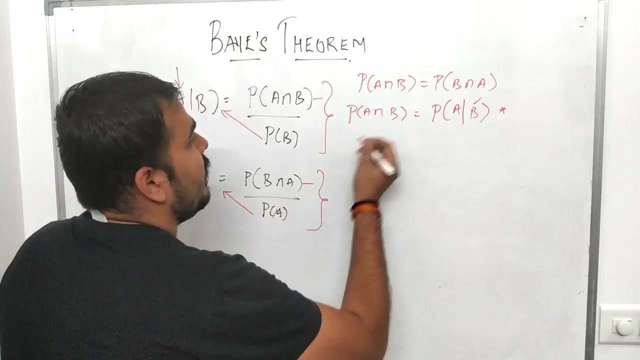 to. You can see that This is nothing but probability of A by B. it is not A by B, A or B. okay. I can also say that probability of A, where we have already given that the probability of B is actually or the B event is actually taken place, okay, multiplied by probability of B and similarly. 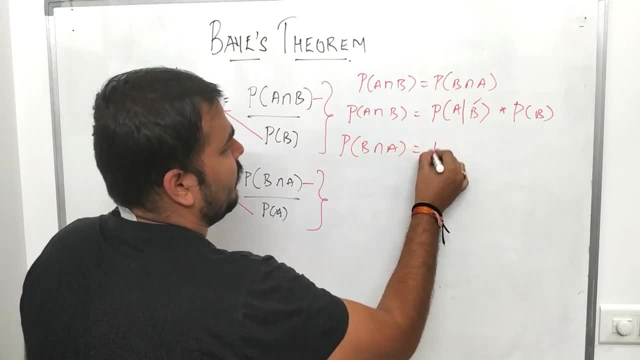 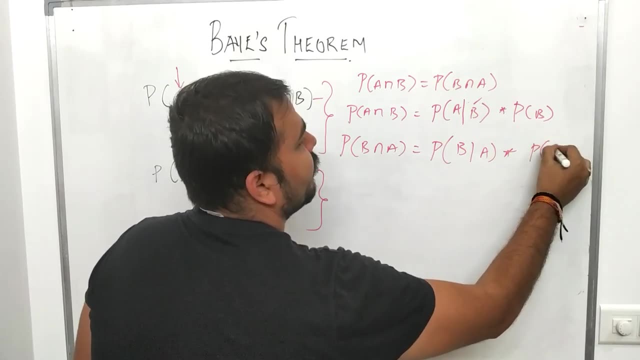 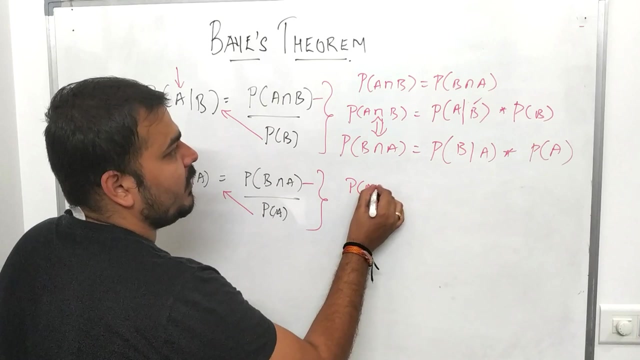 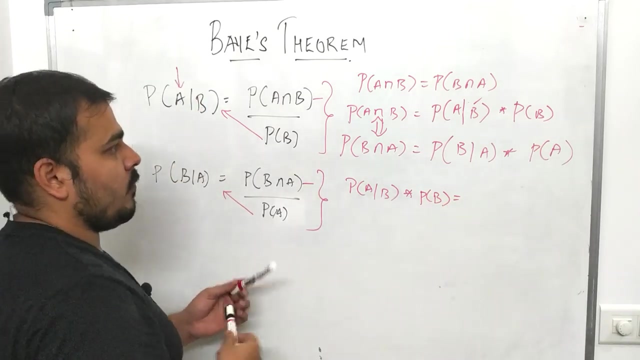 I can write: probability of B intersection A, probability of B where A is given, and this will basically be my probability of A. Now you know that these two are actually equal, so we'll try to equate this and this. so now I can write: probability of A by B multiplied by probability of B is equal to right probability. 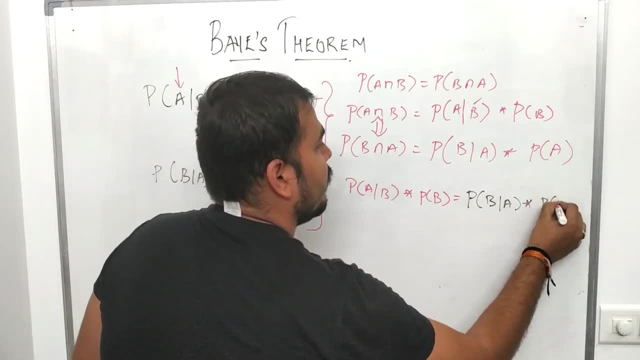 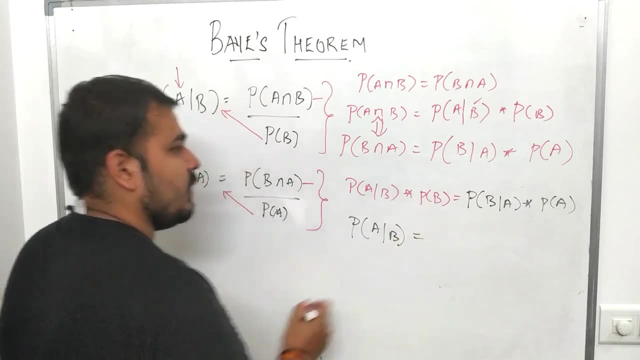 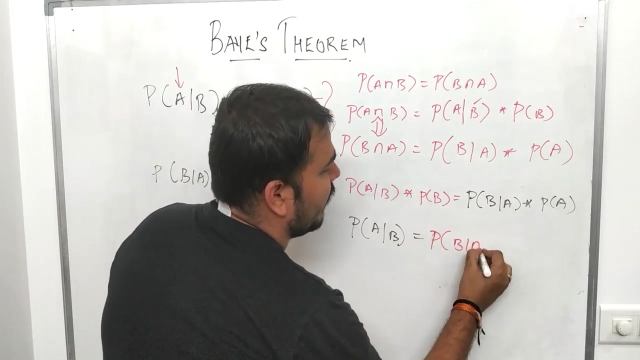 of B by A multiplied by probability of A. right now, if I want to find out what is probability of A by B, Then I can. So, based on the base theorem, I can basically write it as: probability of B bar A multiplied by probability of A divided by probability of B. 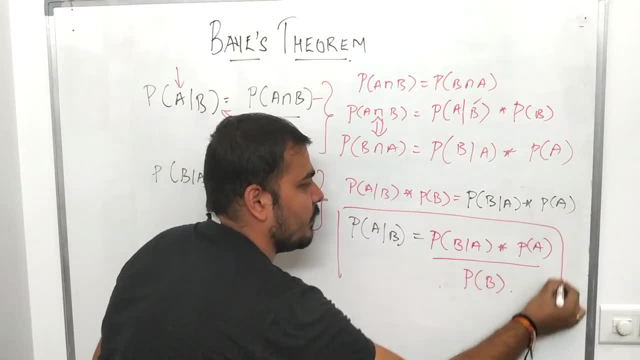 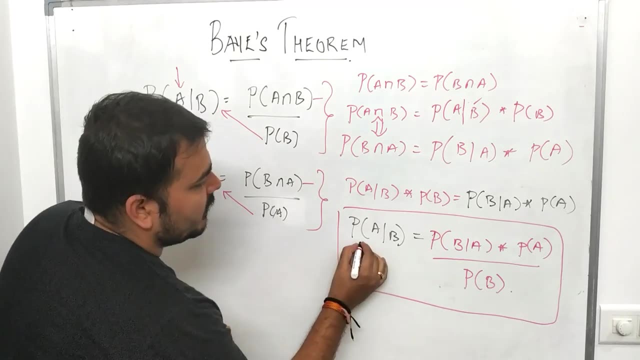 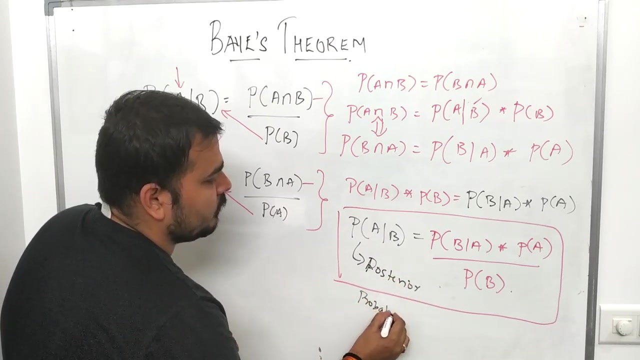 Now we need to understand- and this is this exactly is the base theorem. guys, If you go and try to derive this or see in the internet also, this is actually the base theorem. and remember, this particular value is called as posterior Probability, This is called as likelihood. 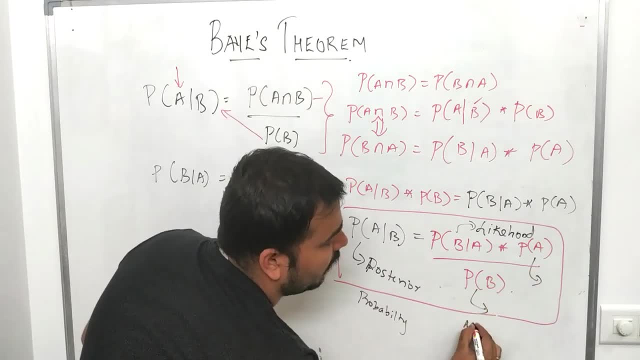 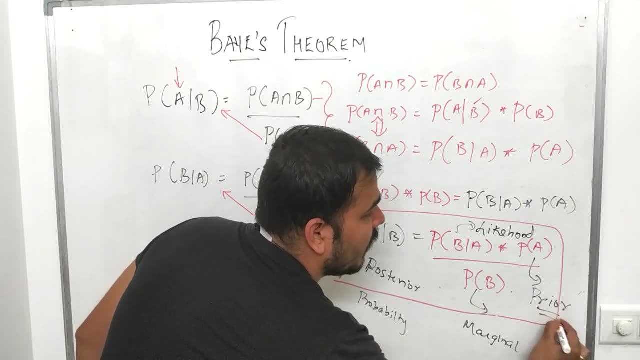 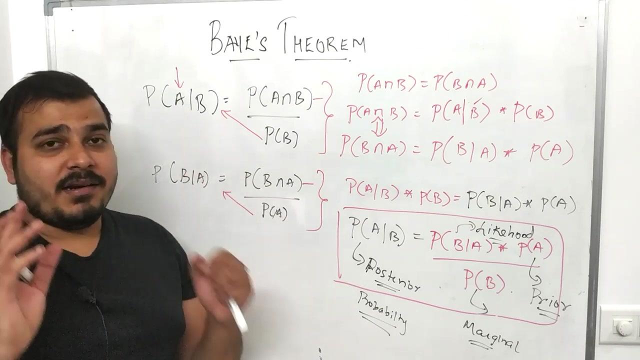 Likelihood probability. this is called as- and this also is called as- marginal probability. okay, and probability of A is called as prior probability. Okay, now, these are the terminologies that are basically used in base theorem. Okay, and we have also seen that. how to derive it? and remember, guys, still I have not told. 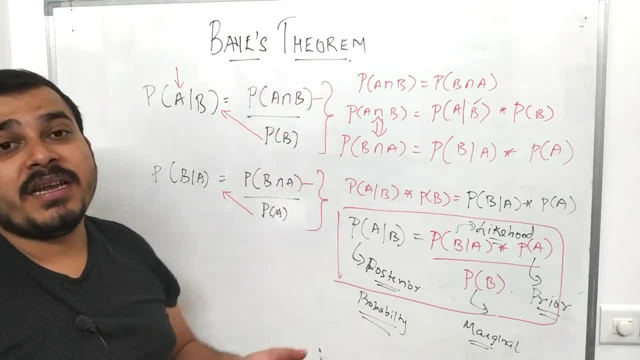 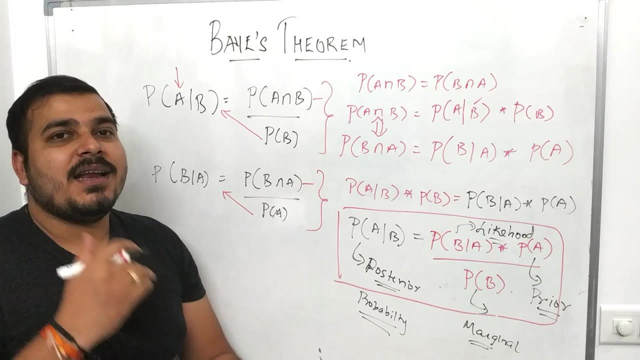 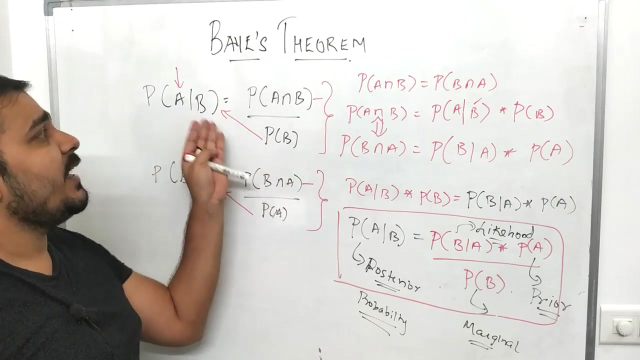 you what exactly and how exactly is Exactly, is base theorem getting used in naive bias classifier? But understand, guys. this particular theorem will help us to easily identify different, different or solve different, different classifications. Understand: naive bias completely works on conditional probability, considering the base theorem in mind.